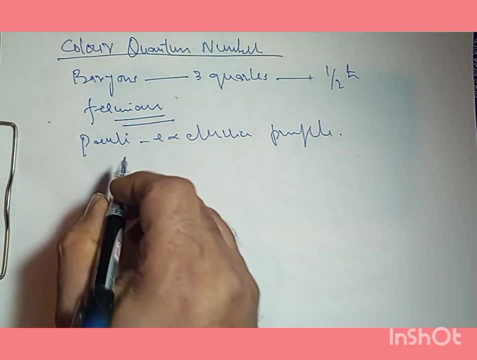 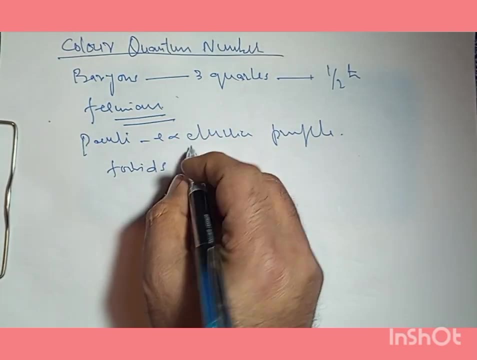 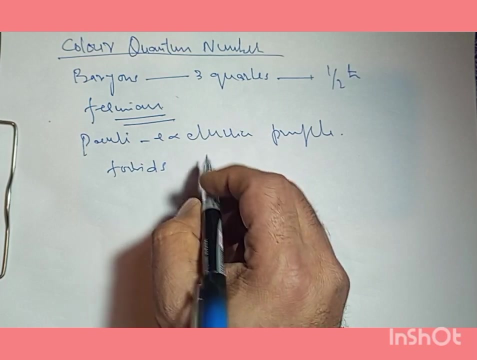 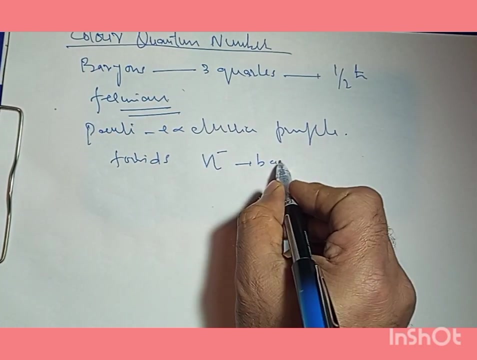 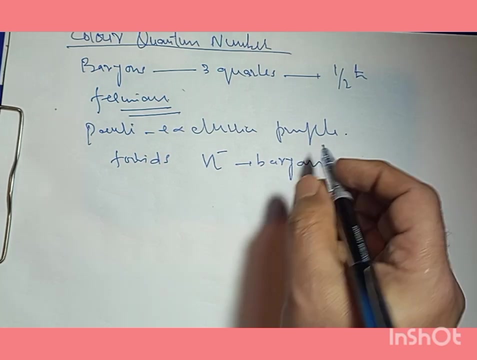 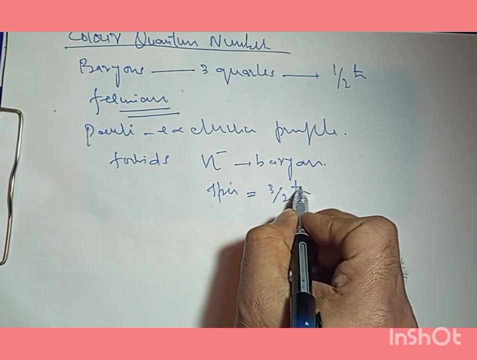 with the same type of corks. It forbids with the same type of corks, or we can say same type of flavor of corks. And considering, if we consider omega minus baryon, if we take this baryon, omega minus baryon, it has a spin. It has a spin of 3 by 2 h h bar. 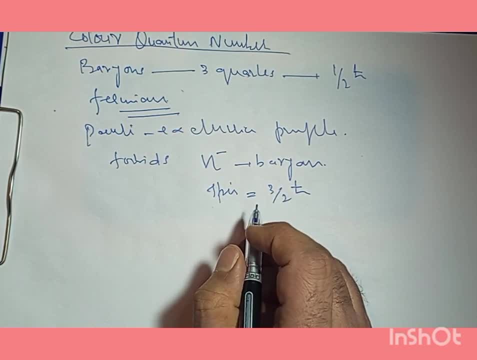 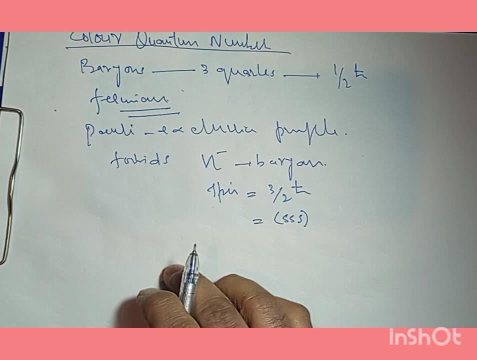 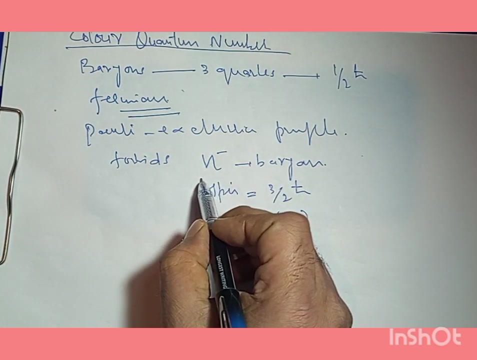 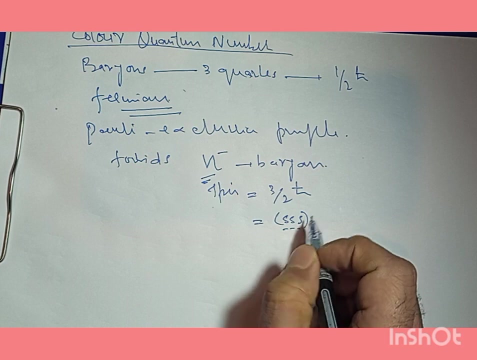 And it's made up of three strange corks And it's made up of S, S, S And S symbolizes the strange cork. Now, According to Pauli's exclusion principle, such particle like this omega negative baryon cannot exist as there are three cogs- S, S and S- constituting like it cannot be in the same state. 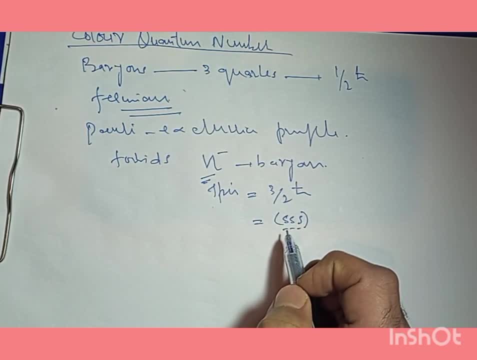 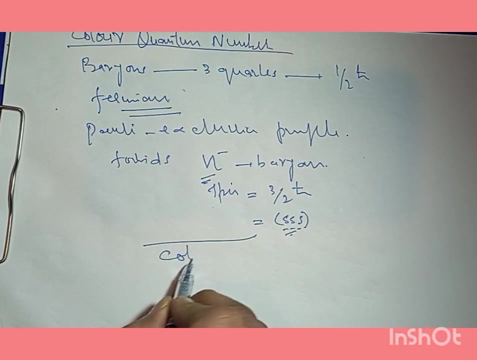 All the three S's cannot have the same state And this problem was resolved by introducing a new quantum number, And this new quantum number or degree of freedom is what is called as color, And this color is required to distinguish the cork which are otherwise identical as S, S and S. 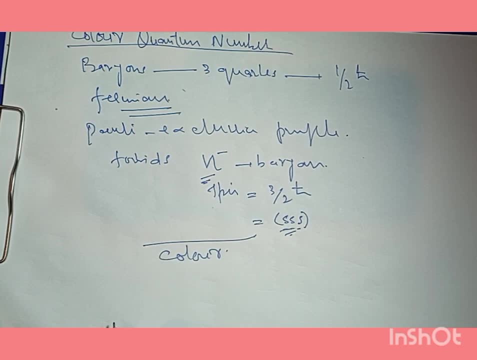 Now it was postulated that corks carry one of the three possible colors, I mean the three possible color quantum numbers. And these three possible colors are: first, one is red R and then the second one is green G. 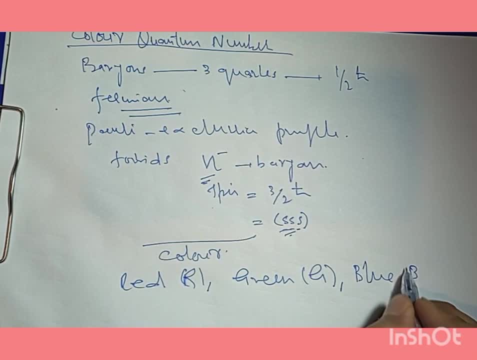 And the third one is blue B, R, G B, And the anti-corks carry the anti-colors. That's, we have anti-red, We have anti-red as R bar, We have anti-green as G bar And we have anti-green. 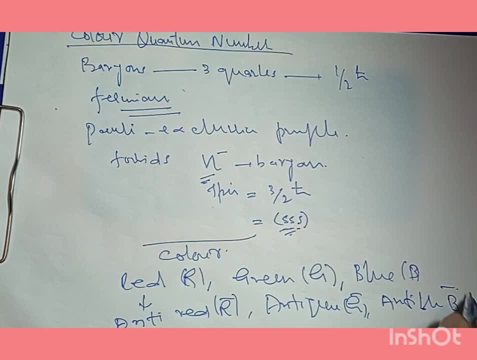 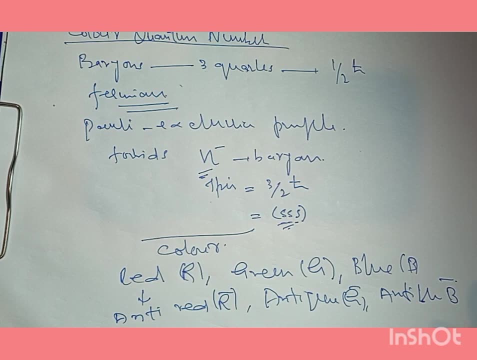 And we have anti-blue as B bar. Now what is important here is that the color quantum number has no relation with actual red, green and blue colors of the visible light, The quantum number. it was named color simply because red, green and blue corks make a colorless state. 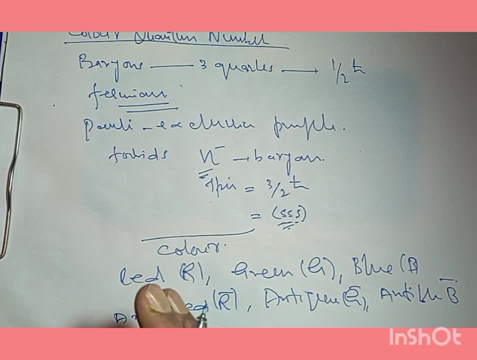 They make a baryon. In the similar way, a white, colorless light is produced due to the mixing of R G, B, due to the mixing of red, blue and green colors of the visible portion of light. Now talking about 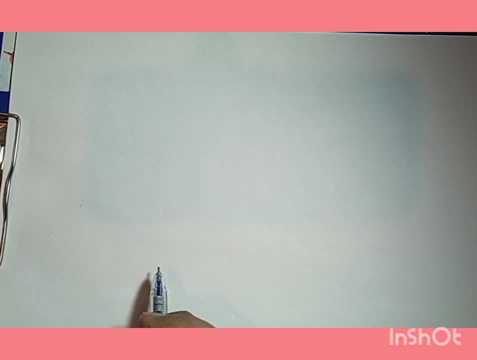 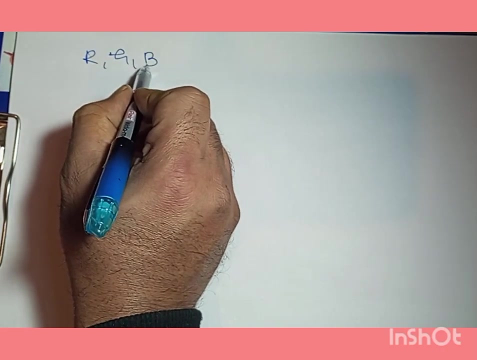 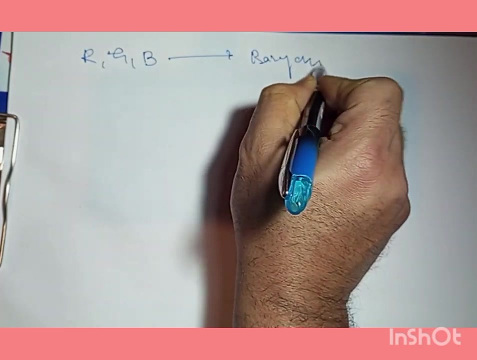 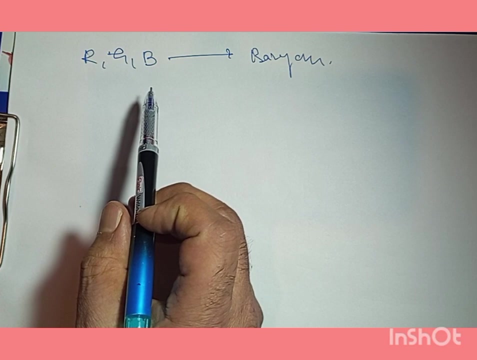 Now, when this red, blue and green corks together make Make a baryon, so this R, G and B corks, they make a baryon. And So what we have is that they make a baryon and the baryon is colorless. 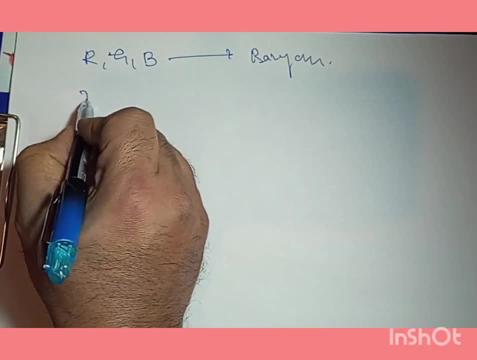 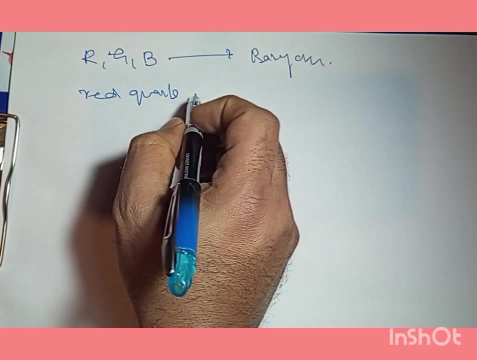 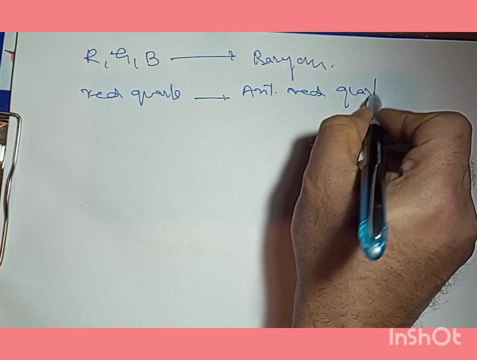 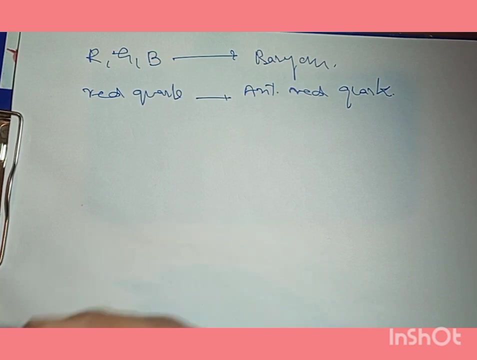 Similarly, the color combination of red cork- If I take red cork, If I take red cork, Red cork and anti-red cork and anti-red cork. and the color combination of blue cork and anti-blue cork and green cork and anti-green cork. 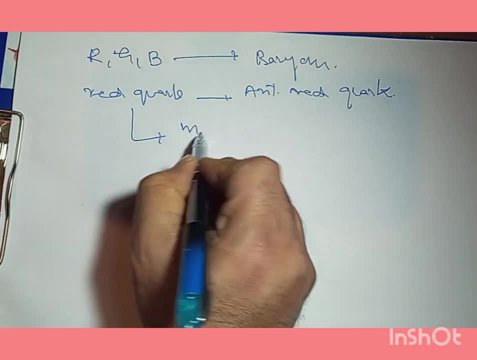 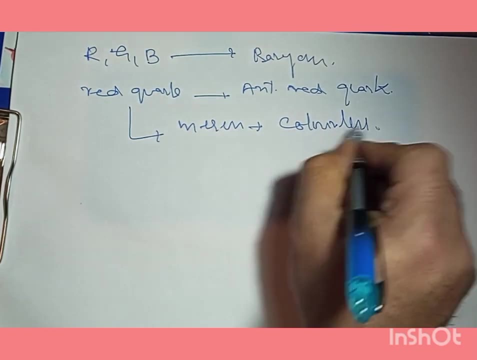 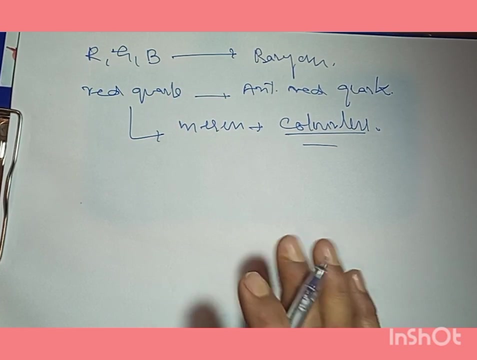 what they do is they all make massons, And these massons are colorless. They don't have any color. Now, in the beginning, color quantum number was introduced to solve the theoretical problem of cork model, But later on, its real existence. 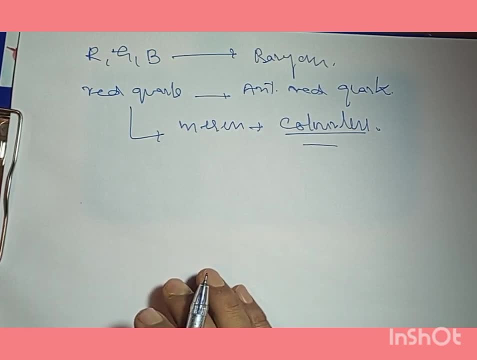 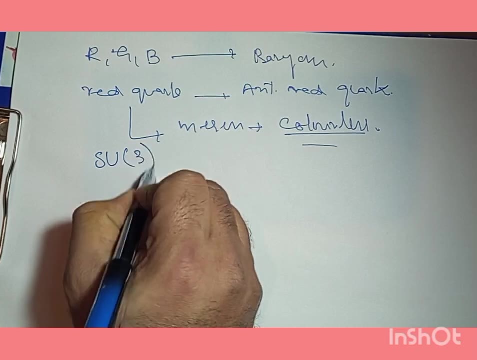 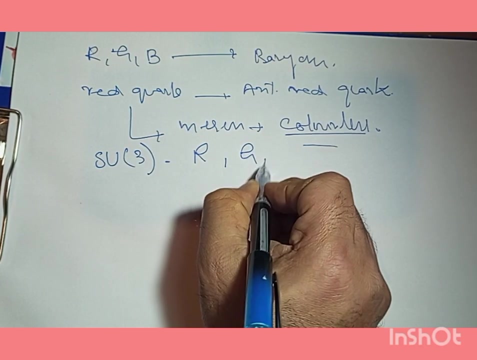 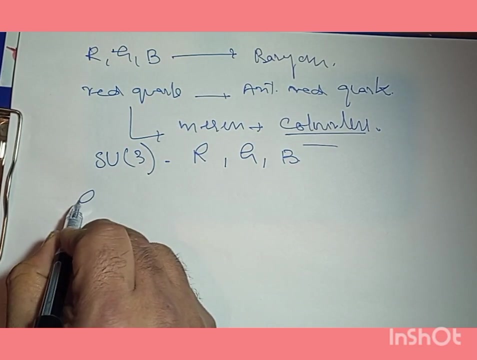 The real existence of the color of the cork was established experimentally. Now, if we talk about, There's a formula called Sucr-3.. And take R as red, G as green cork and B as blue color states, And this R, this red state, is 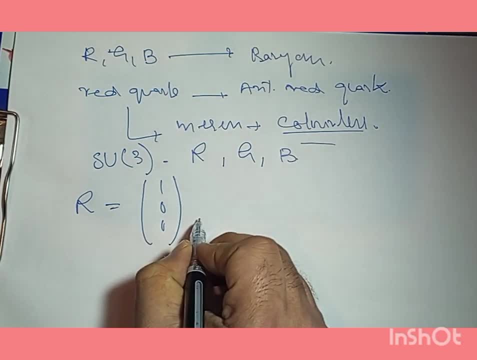 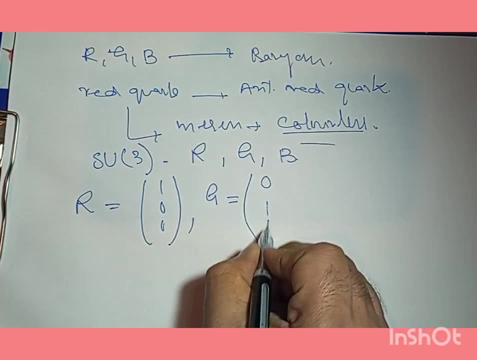 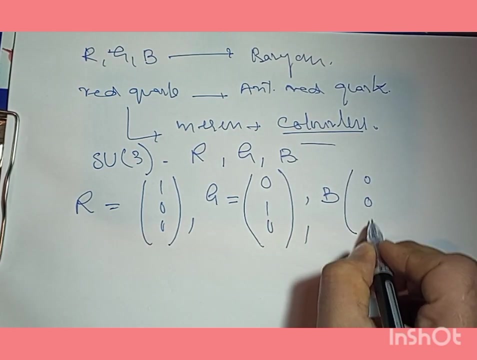 is a matrix: 1, 0, 0.. And this, This G, This G color state is. This G color state is is 0 1 0 and this blue color state is 0 0 1. now the color states have have two quantum numbers. 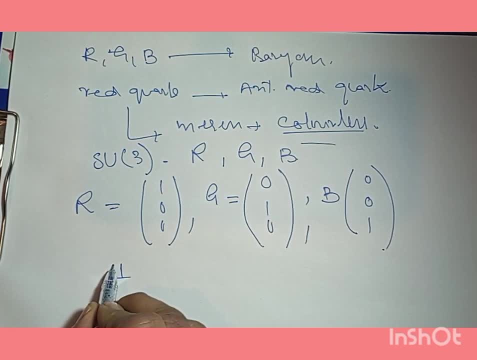 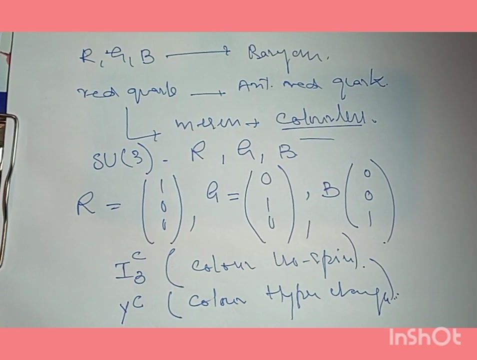 and we have here i3 c and, and this is the color iso spin, this is the color iso spin, and y c, and this is color hypercharge, color hypercharge. now let's, let's tabulate uh, the, uh, these, these color, uh, color states of a cork. 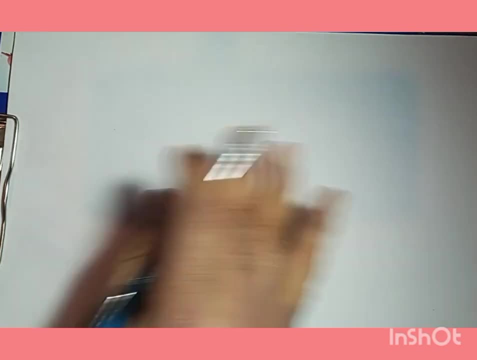 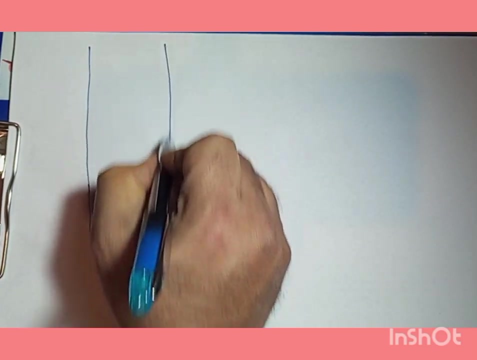 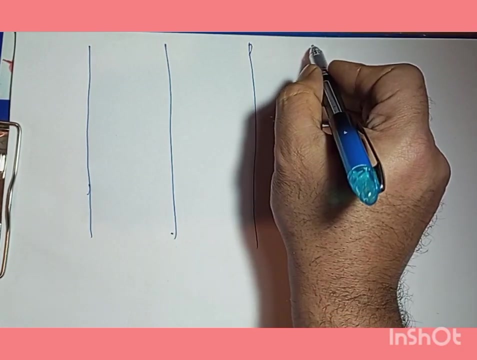 and what we will do is we will use this color hypercharge and we will use this color hypercharge we will have here is, we will have the color state and then we will take the iso spin, we will take the hypercharge and and then again we'll go with the, with the color state of. 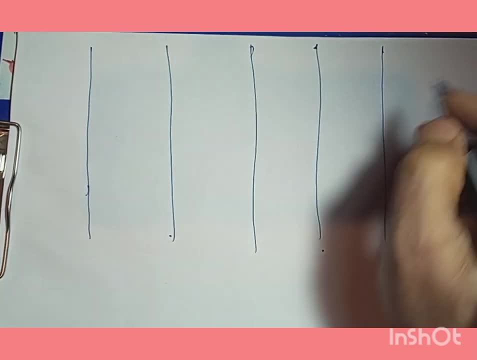 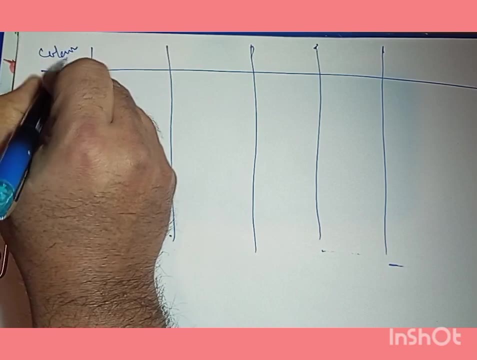 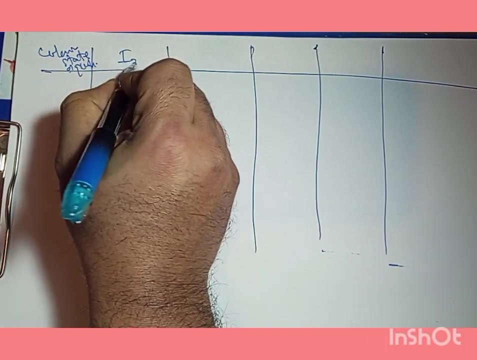 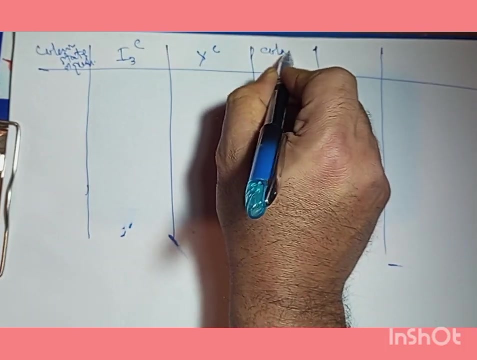 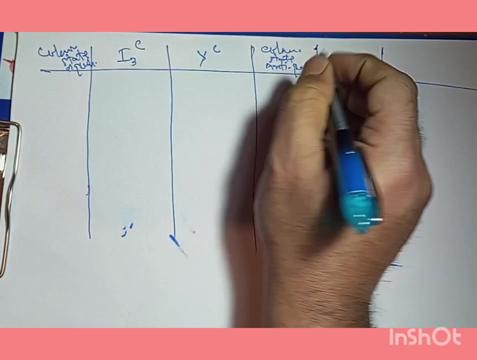 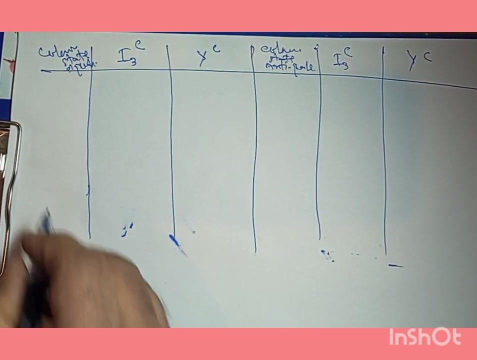 anti-cork, then their iso spin and hypercharge. so let's go with that. so here i have color state of cork. the color state of cork now i3c, it's iso spin, it's hypercharge. then the color state of anti-cork, anti-cork- then it's iso spin and hypercharge. okay, so the first one. 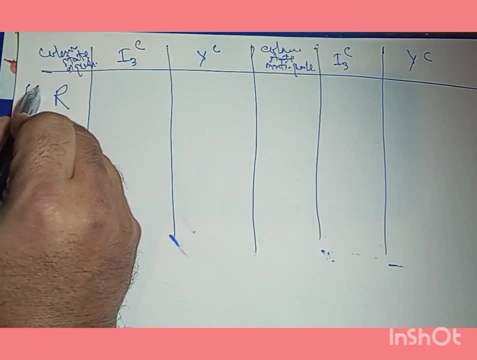 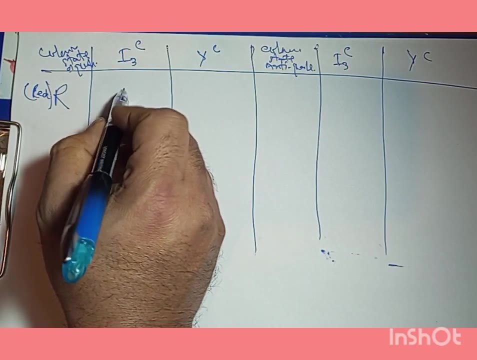 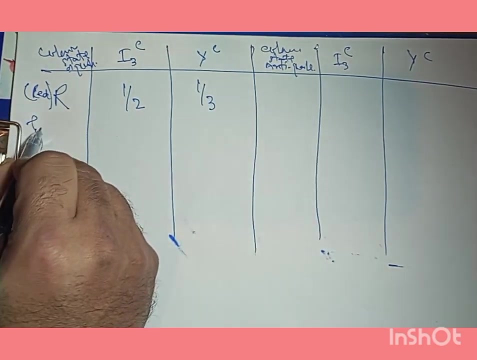 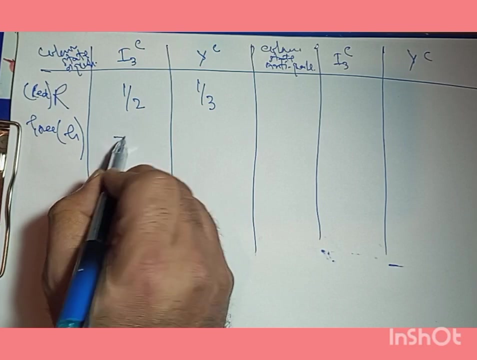 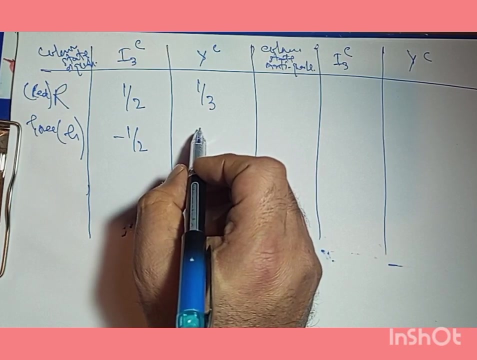 is is red, uh, and this is red. i should write red red color. and it has: i3 is half, its hypercharge is one by three and green g: uh, it's, uh, it's. i3c is minus half and it's uh. its y is is its hypercharge. 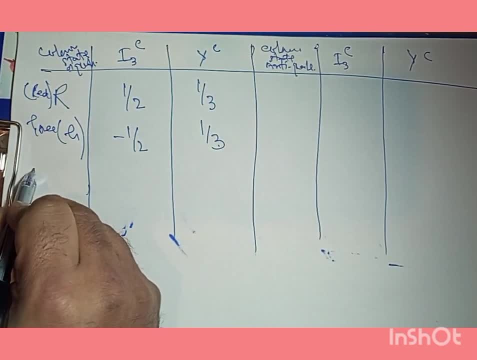 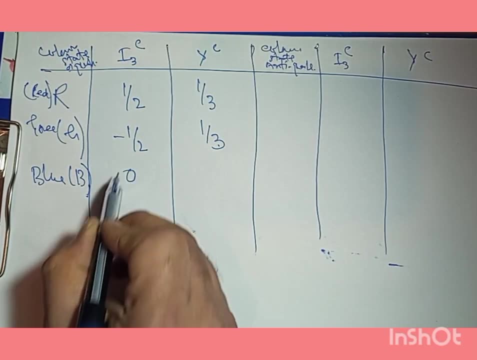 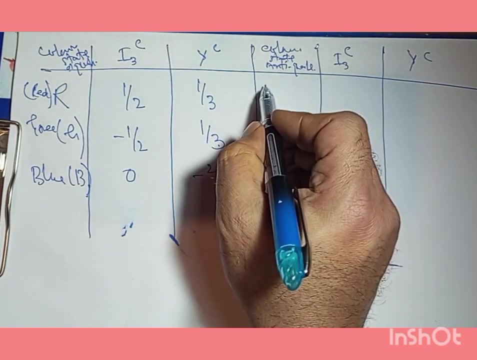 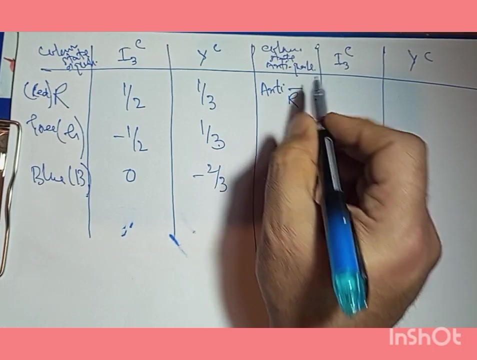 charge is 1 by 3. and then we have blue, that's B cork, and it has 0 I 3 and it has minus 2 by 3, a hypercharged state then going with anti, so this will represent anti, so anti red is our bar, so it has. it has ISO spin of minus half and 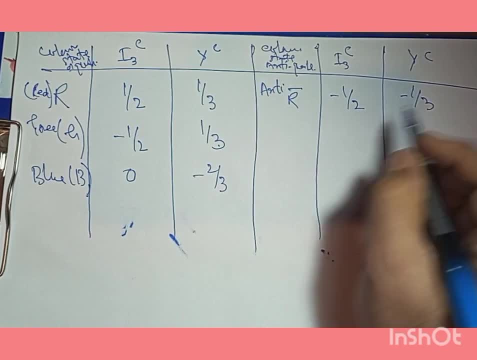 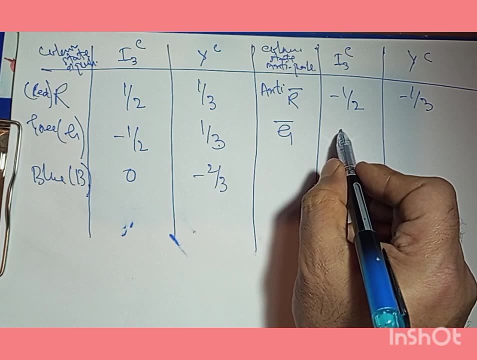 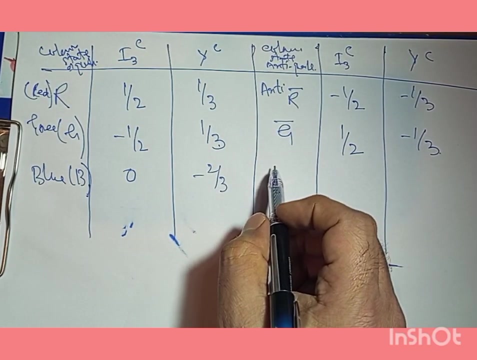 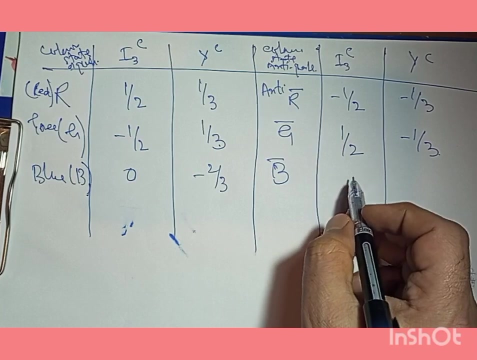 it has hypercharge of minus 1 by 3. and then we have anti green, that's G bar. it has I 3, that's 1 half, and minus 1 by 3 is its hypercharge. and and finally, what we have here is is blue B bar, and for B bar, what we have I 3 is 0 and it's 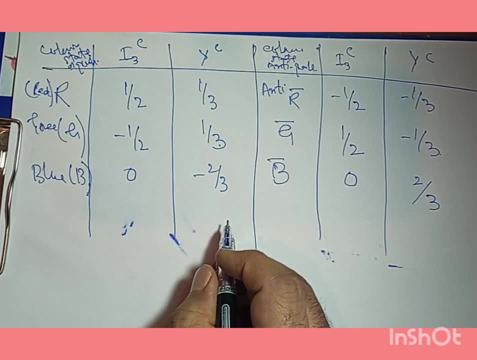 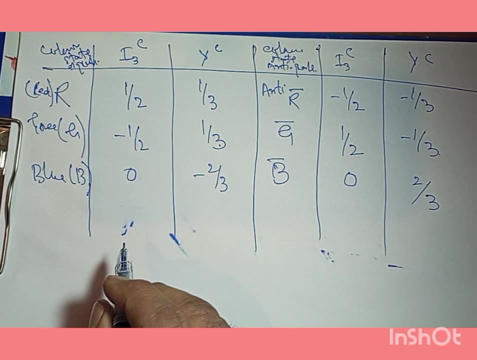 hypercharge is minus 1 by 3. and then we have anti green, that's G bar, and it has is is 2, its hypercharge is 2 by 3. so this is this is how we can, we can summarize, we can table it: these, these color quantum numbers, the these, these, 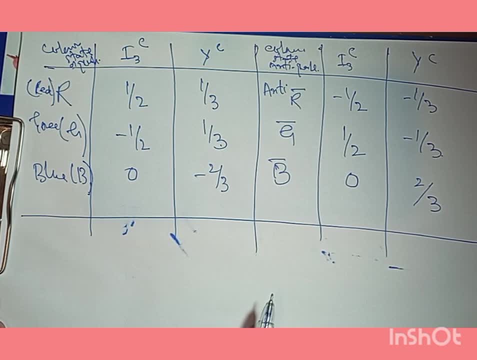 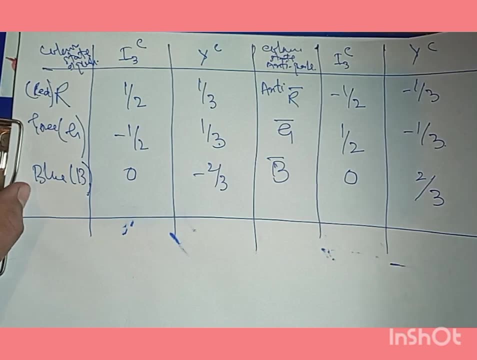 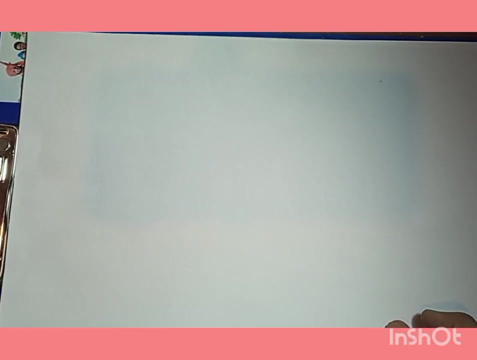 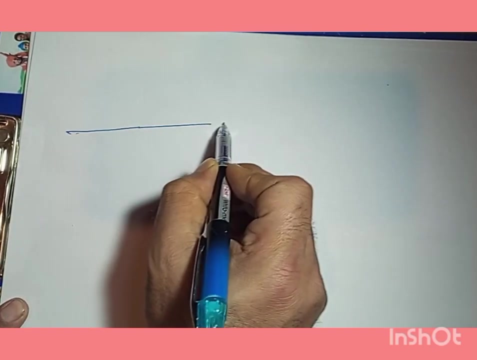 color color cogs, color states of of the cogs. now let's go with the, with the weighted diagram of, with a diagram of of these color cogs and anti color cogs. now for. so weighted diagram we have in terms of, we have in terms of I 3- okay, I suspend- and in terms of hyper charge and 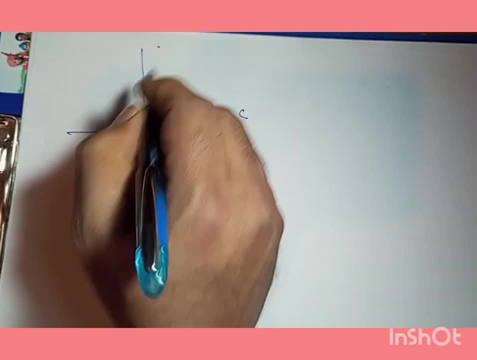 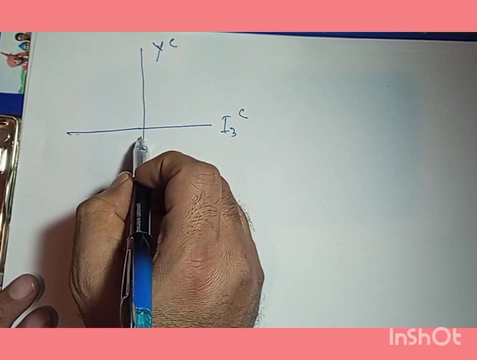 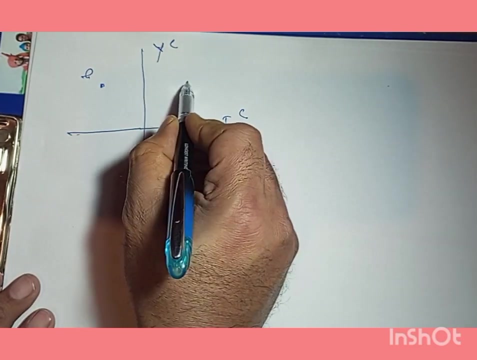 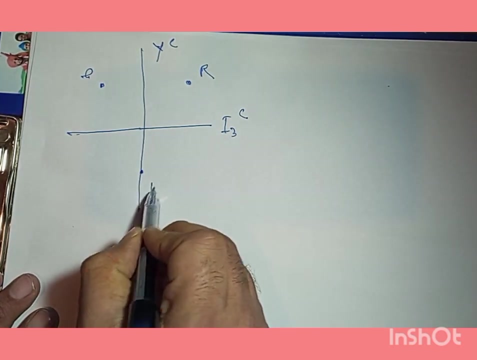 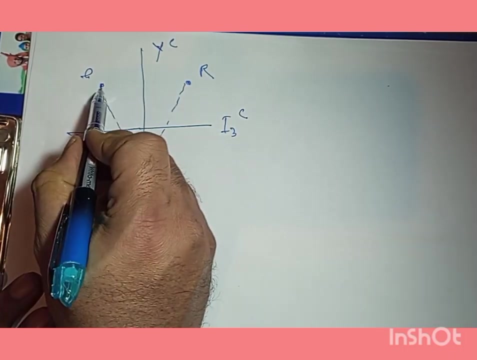 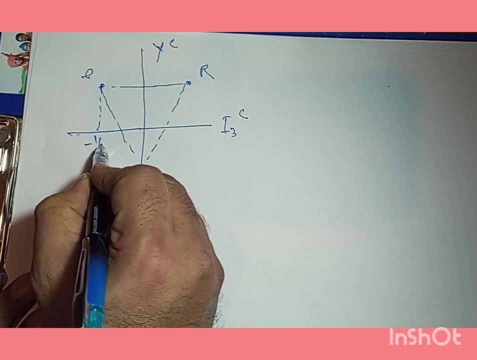 hyper charge we have. we have Y, raised power C, so this will be a representative of my, of my cogs. so here I have G, and here I have R, and and here I have B, so so I would like to join them and and and this: this is my minus half for isospin and 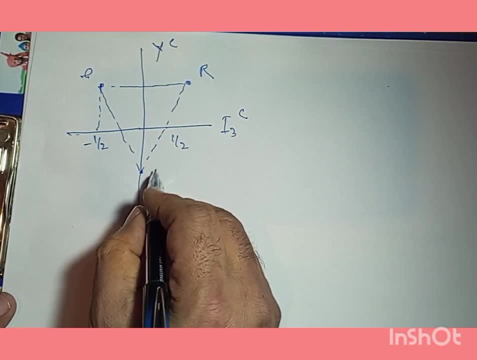 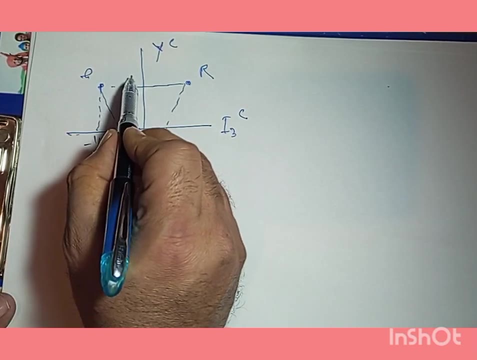 this is my minus half for isospin, and and this will be plus half, and and this will, this will be plus half, and and this will be minus 2 by 3 hypercharge for blue and be minus 2 by 3 hypercharge for blue, and here they will have 1 by 3 about green. 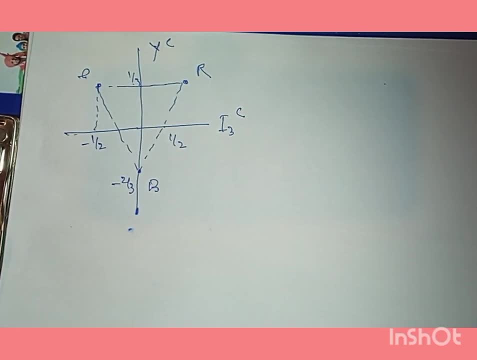 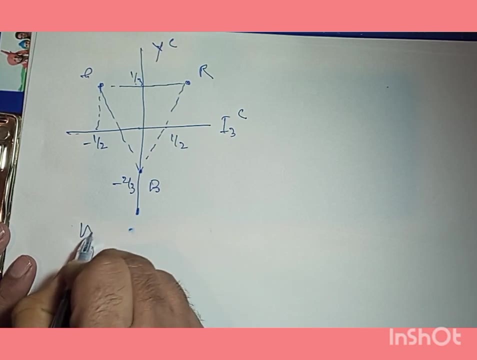 here they will have 1 by 3 about green and green and red. now let's go with the and red. now let's go with the weighted diagram of the anti color cogs. so this weighted diagram of the anti color cogs, so this is the weighted diagram, weighted. 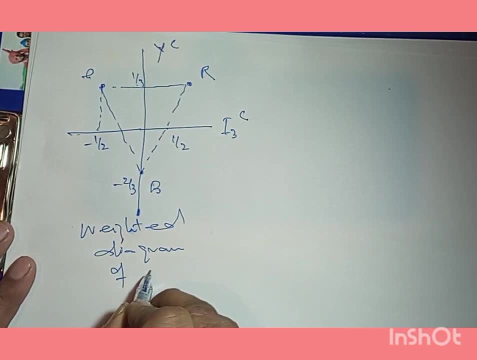 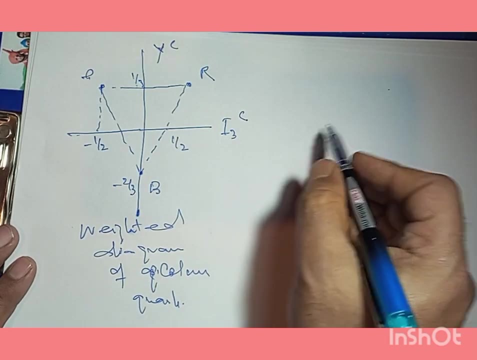 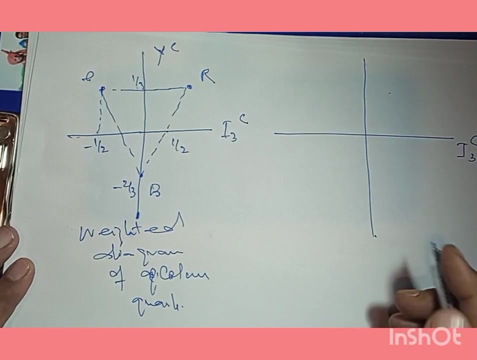 is the weighted diagram. weighted diagram of corks- color corks- sorry, color corks. and and looking for its anti. so this is isospin, so this is i3c and this is hypercharge. so let us invert it. so this is going to give me g. 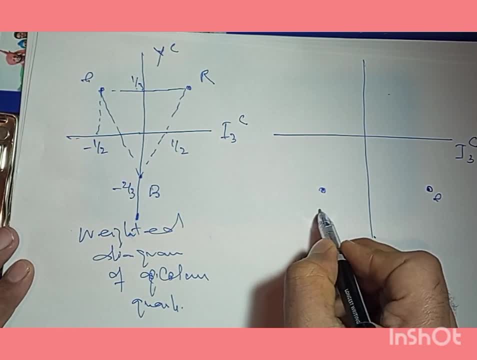 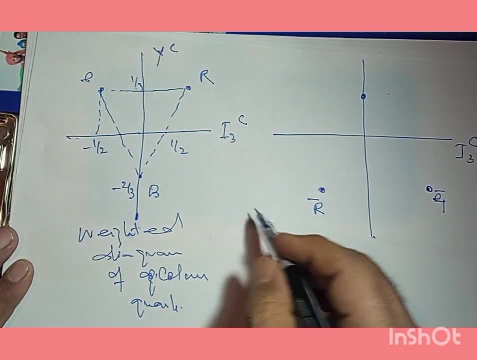 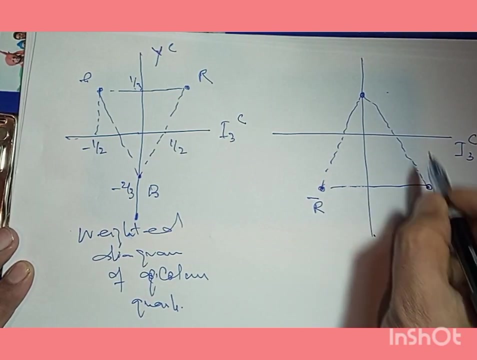 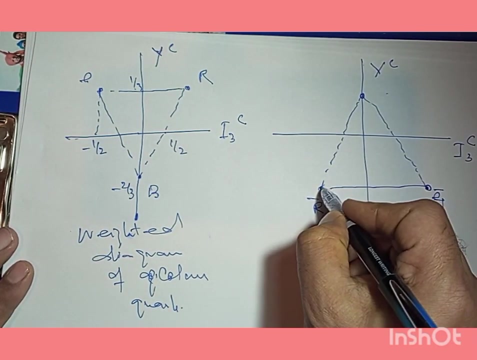 and this is going to give me r. they have to be bars, bars, and, and this is going to be my b bar, so let's join them. so this is the hypercharge. that's y c. okay, so this will be my minus half and this will be my minus half, and this will be my minus half and this will be my minus half. 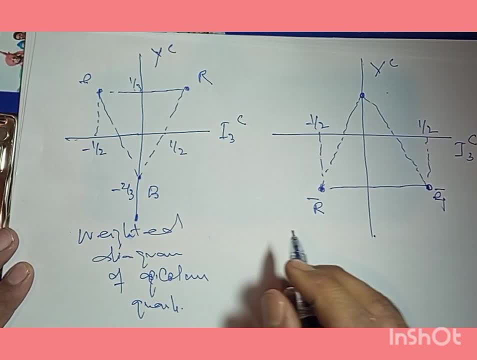 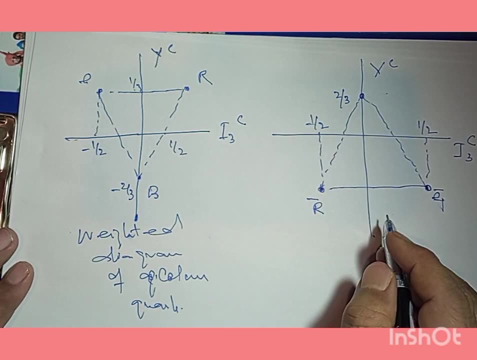 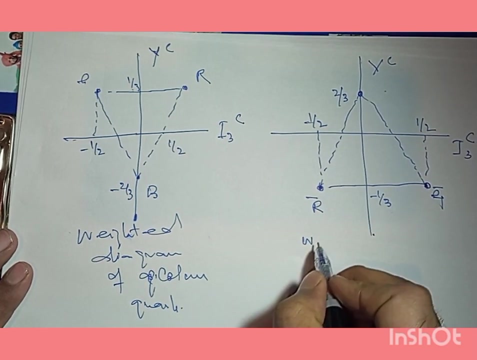 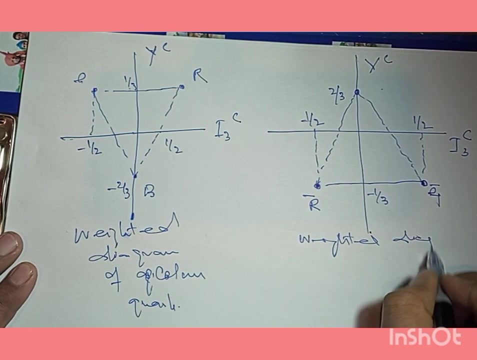 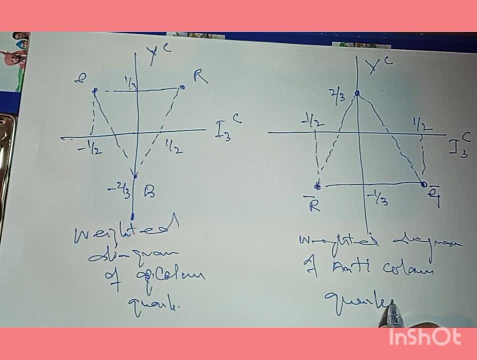 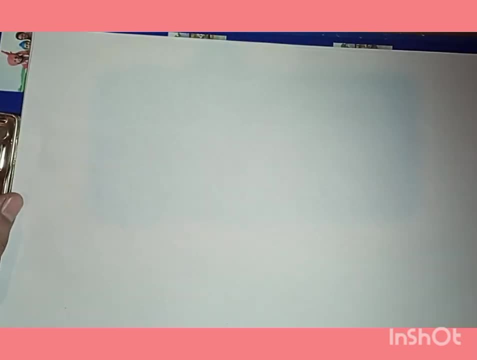 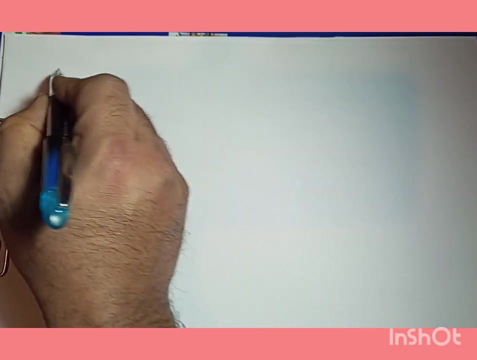 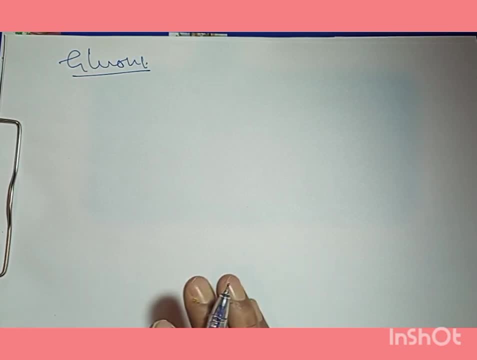 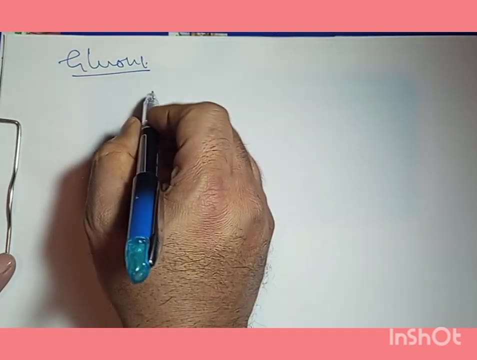 blue ones, now blue ones. basically blue ones, now blue ones. basically, basically the corks constitute hadrons, basically the corks constitute hadrons, basically the corks constitute hadrons. and these corks inside the hadron, uh, what they do is they interact through, through the exchange of gluons. 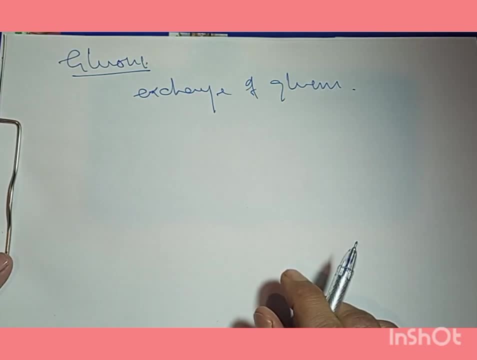 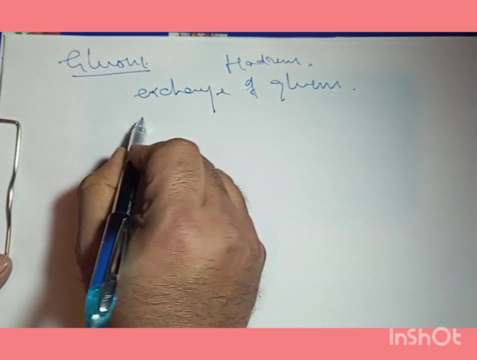 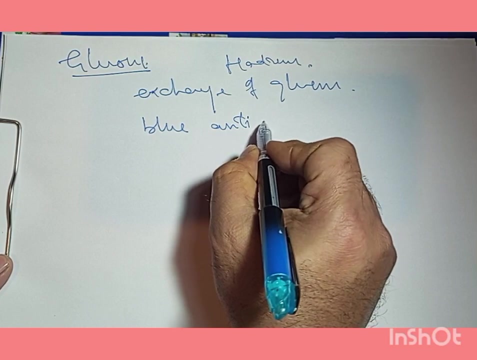 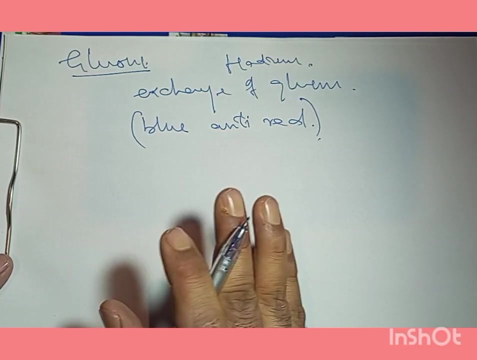 exchange of gluons in hadrons. okay, exchange of exchange of gluons. now, each gluon has a color and anti-color combination, for example, blue, uh and anti-red. that allows it it to transmit color when, when exchange it with each other. now, now the color is. 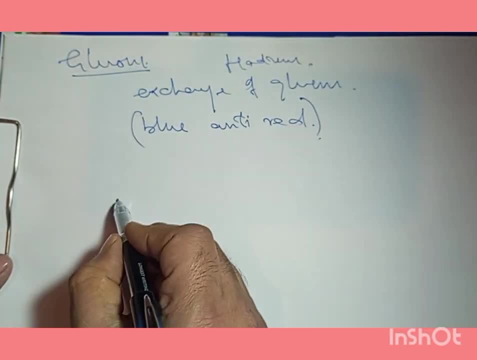 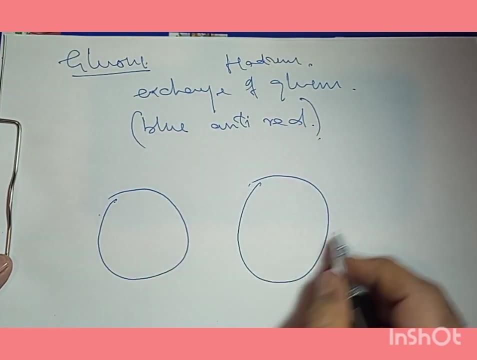 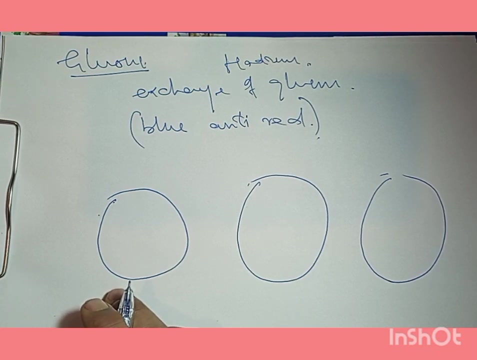 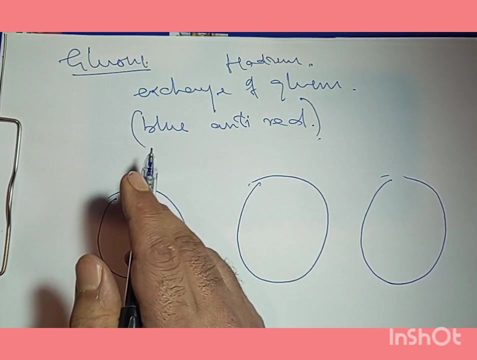 is conserved during the emission and the absorption. so so if i take some- uh, if i take some, some sort of example to understand this now, what i have here is that that the color is conserved during the emission and absorption of these gluons, and these gluons are exchanged. 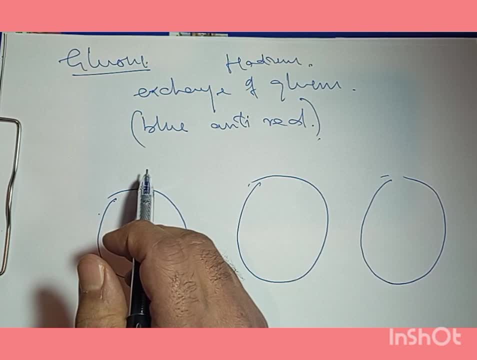 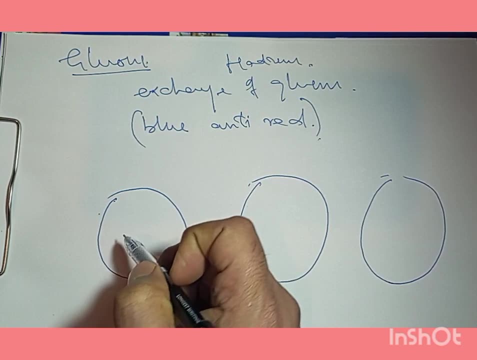 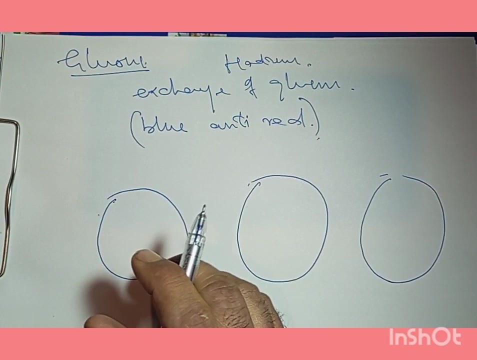 between between the cogs and the process of exchange of gluon changes the color of the cork continuously with respect to the exchange of gluons. now, talking about meson say, for example, meson is made up of a cork and anti-cork. okay, the color of